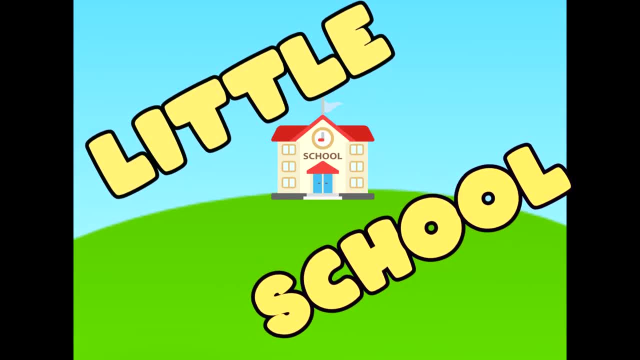 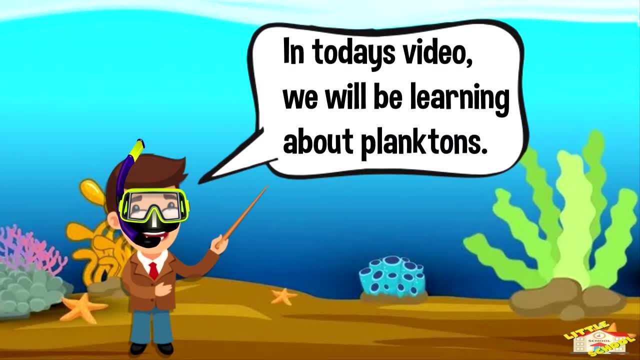 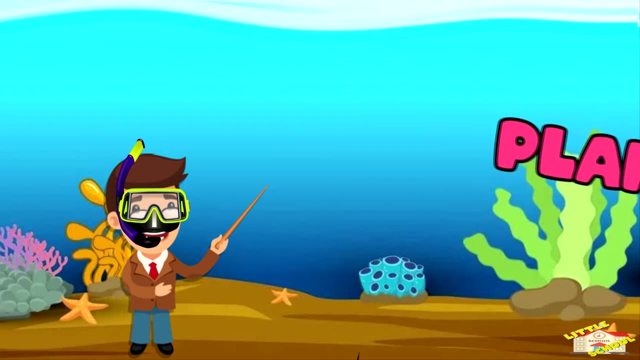 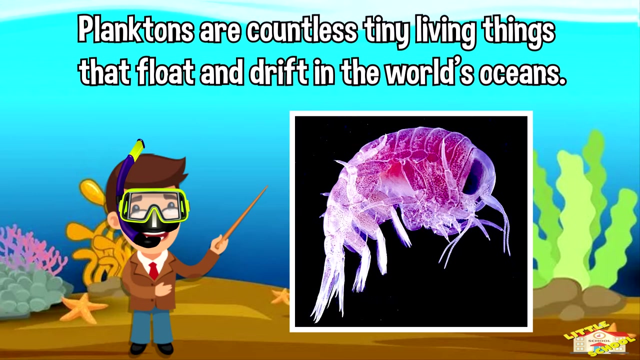 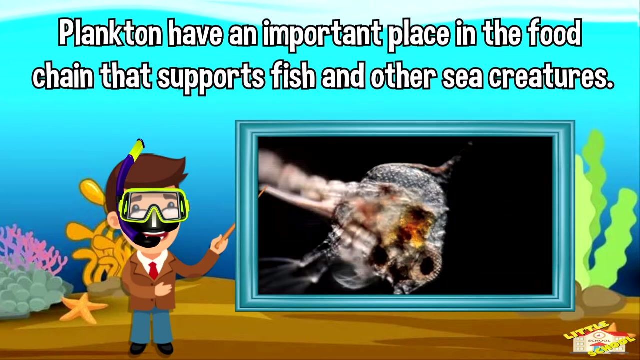 Hey kids, In today's video we'll be learning about planktons. Are you ready? Let's begin. Planktons are countless tiny living things that float and drift in the world's oceans. Planktons have an important place in the food chain that supports fish and other sea creatures. 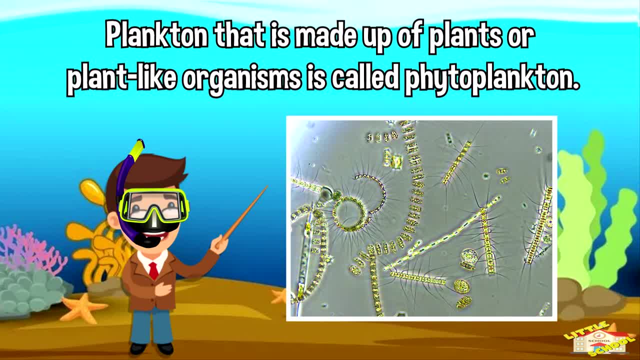 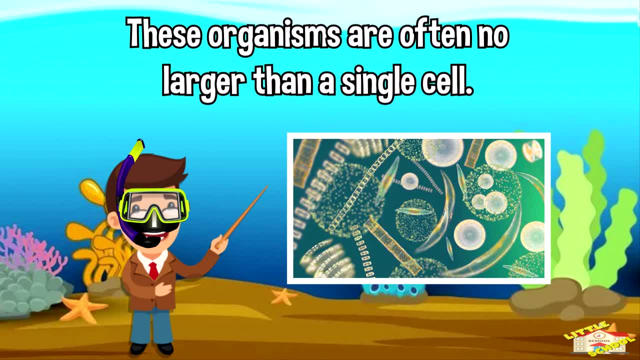 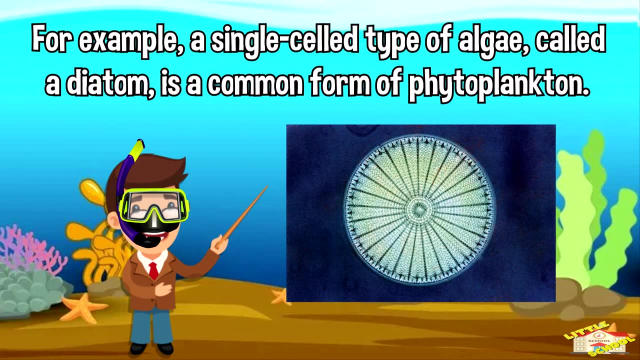 Plankton that is made up of plants or plant-like organisms is called phytoplankton. These organisms are often no larger than a single cell. For example, a single-celled type of algae called a diatom is a common form of phytoplankton. Phytoplankton floats near the surface of the 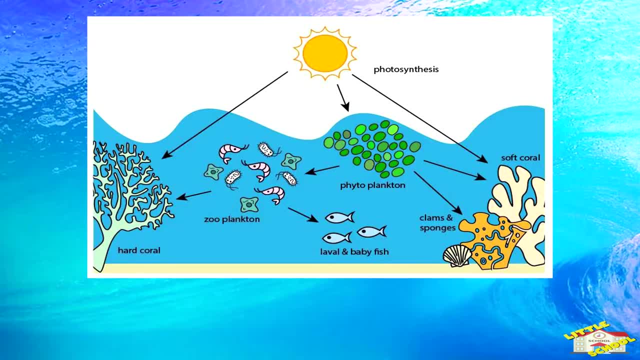 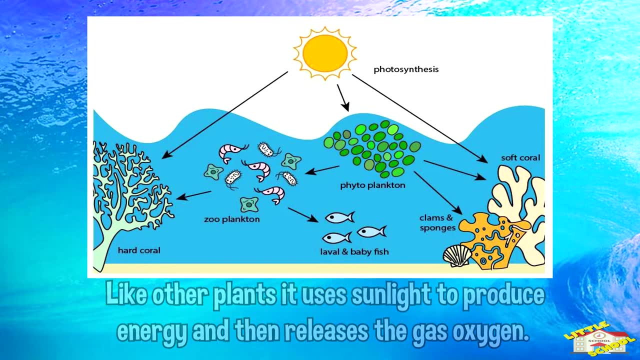 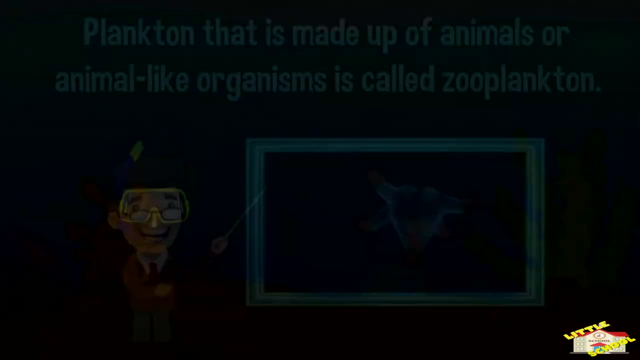 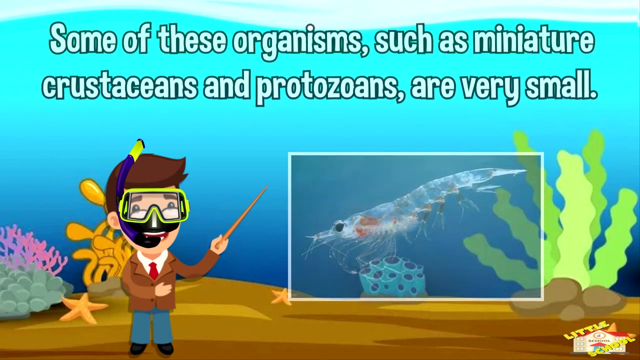 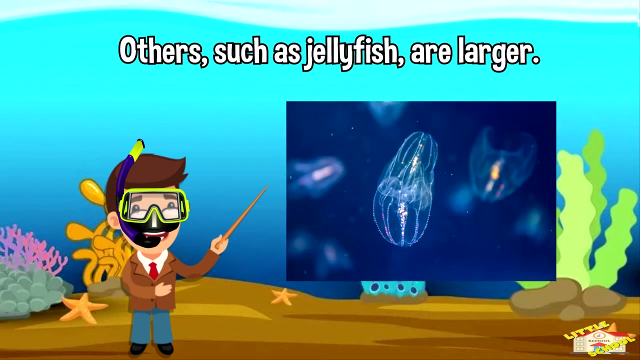 water. Like other plants, it uses sunlight to produce energy and then releases the gas oxygen. This process is called photosynthesis. Plankton that is made up of animals or animal-like organisms is called phytoplankton. Some of these organisms, such as miniature crustaceans and protozoans, are very small. 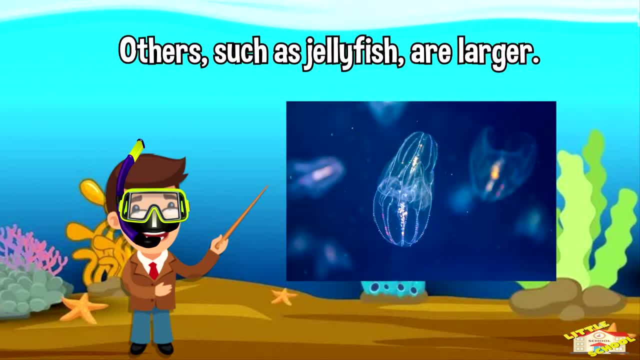 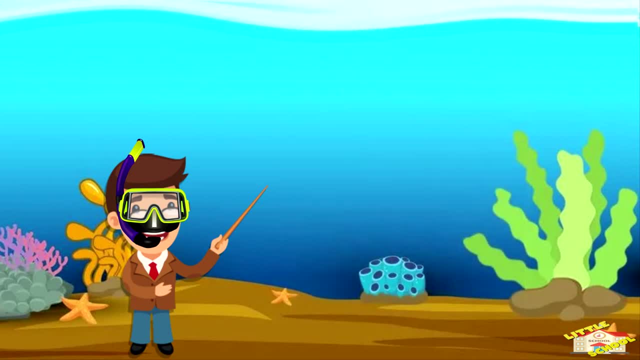 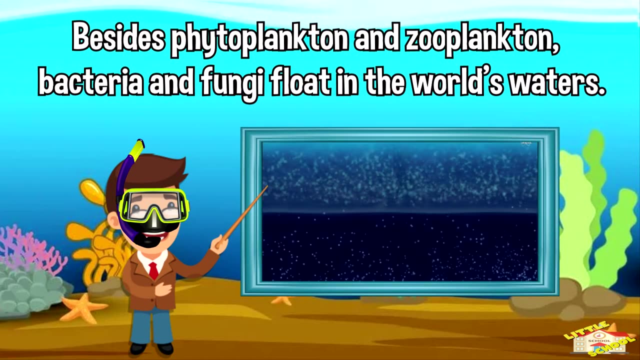 Others, such as jellyfish, are larger. Some fishes and shellfish begin their lives as eggs or tiny larvae. These eggs and larvae are also zooplankton. Besides phytoplankton and zooplankton, bacteria and fungi are also found in phytoplankton. Phytoplankton is a 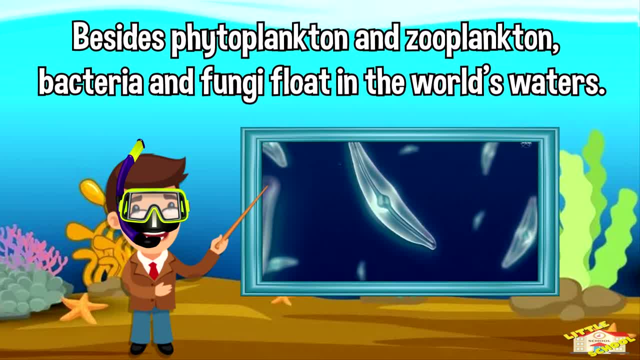 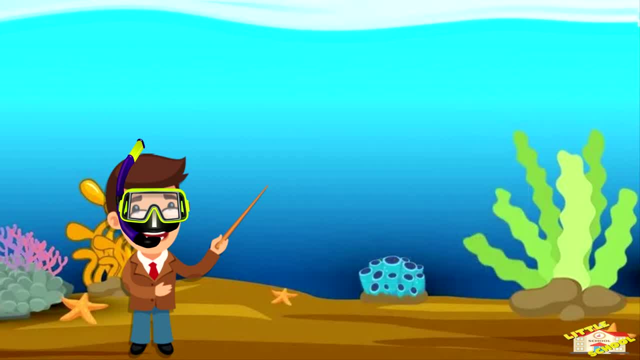 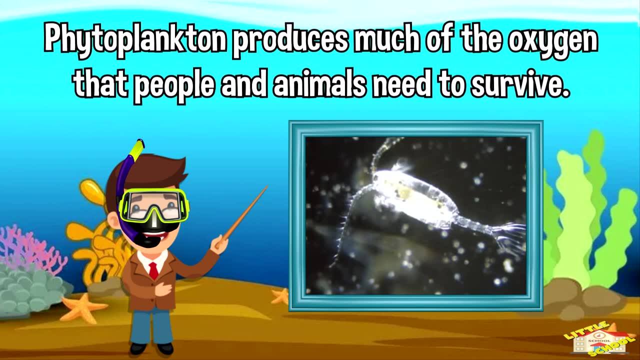 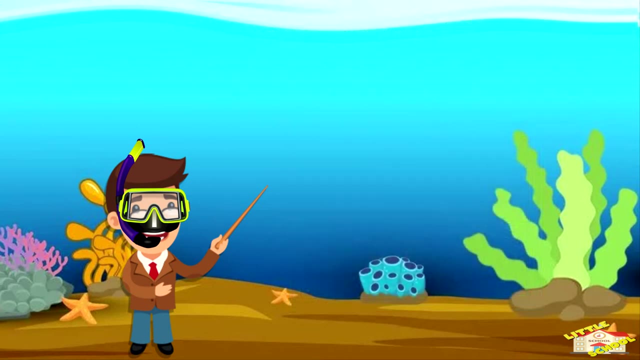 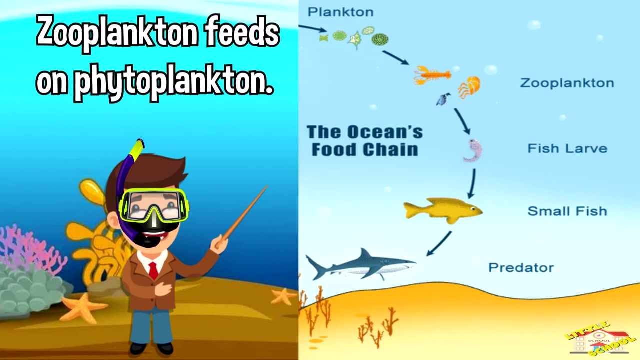 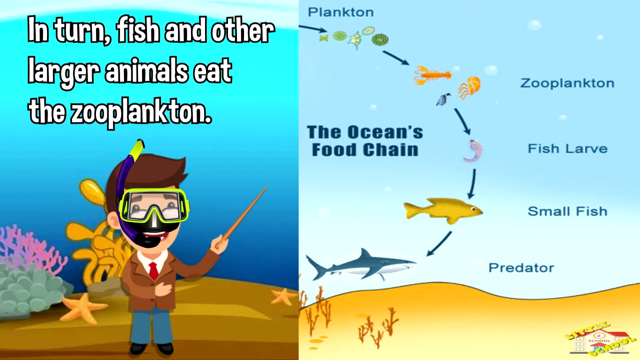 primary source of herbivores and verdurans, Phytoplankton produces much of the oxygen that people and animals need to survive. Fol worksheet 208. Zooplankton feeds on phytoplankton. In turn, fish and other larger animals eat the zooplankton.